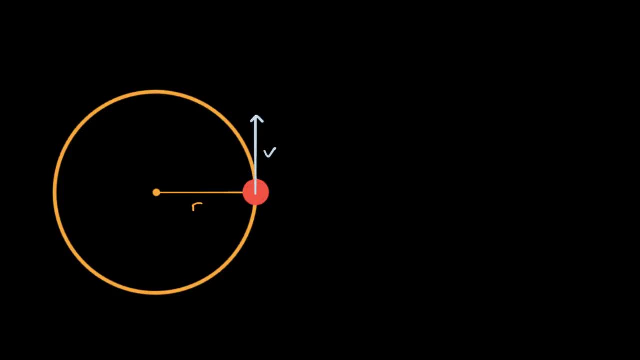 So even if I have the same speed at this point as I have, at say, this point right over here, my velocity will be pointing in a different direction. So now the magnitude might be the same. I'll try to draw it roughly- that same. 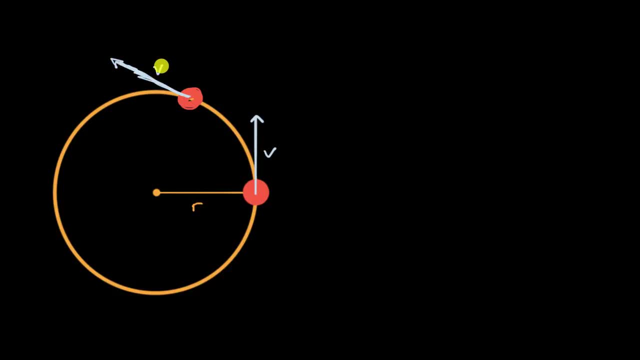 the length of this arrow should be the same, So the magnitude v. without an arrow on top, you could view that as the linear speed. that will be the same, but now the direction has changed. And in order to change the direction, 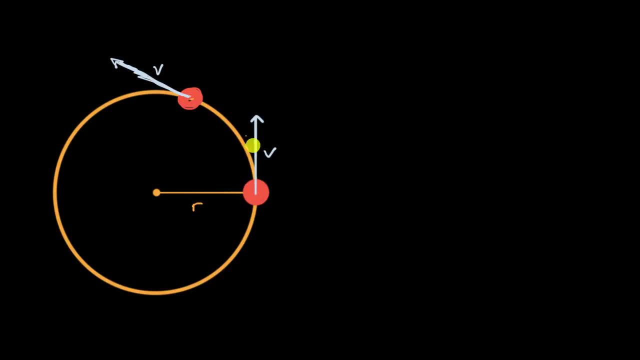 you must have this ball that's moving in. this circular motion must be accelerated. That's the only way. if you have a change in velocity, then you must have acceleration. And it's a little counterintuitive at first because you're saying: well, my magnitude didn't change. 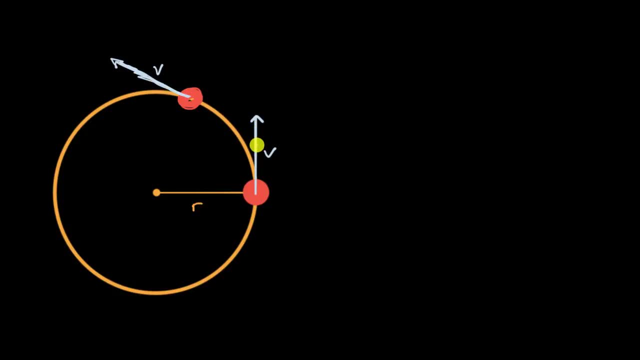 only my direction did. But any change in your velocity implies an acceleration And in previous videos we saw that that acceleration is constantly going to be inward. if you have your uniform circular motion, And we call that inward acceleration, we call that centripetal acceleration. 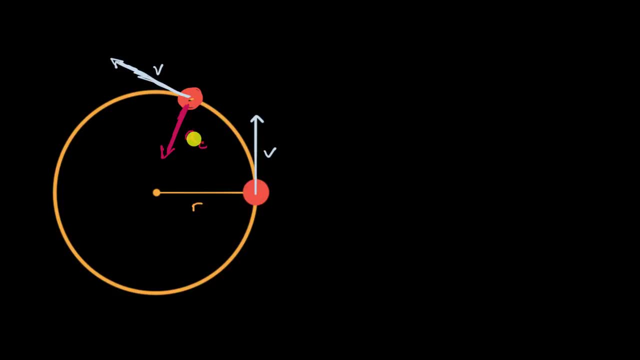 And though, if I write it without, if I write this, a sub c like this, this means the magnitude of my acceleration. and if I write it without, if I write this a sub c like this, this means the magnitude of my centripetal acceleration. 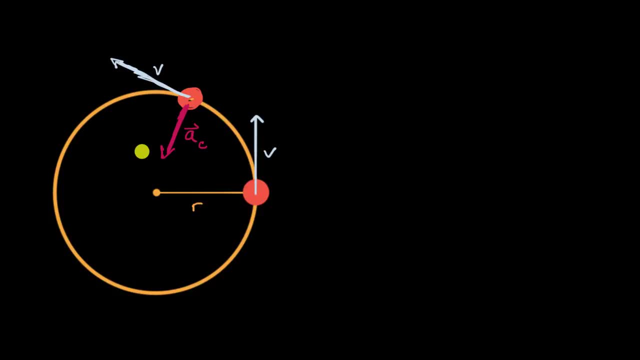 If I'm talking about the magnitude and the direction, I would put an arrow on it just like that. Now we have also in previous videos, have been able to connect. what is the magnitude of centripetal acceleration? how can we figure that out? 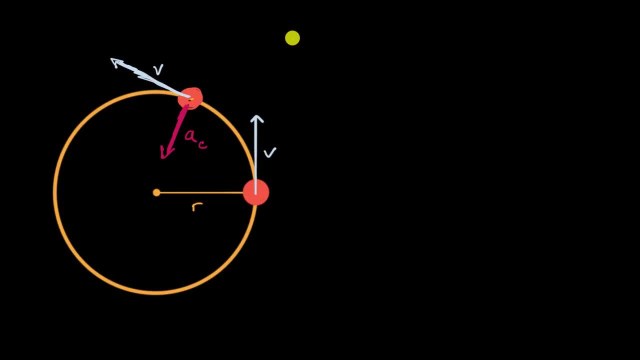 from our linear speed and the radius, And we had the formula: the magnitude of centripetal acceleration is equal to the magnitude of our velocity or our linear speed, squared divided by, divided by our radius. Now what I wanna do in this video? 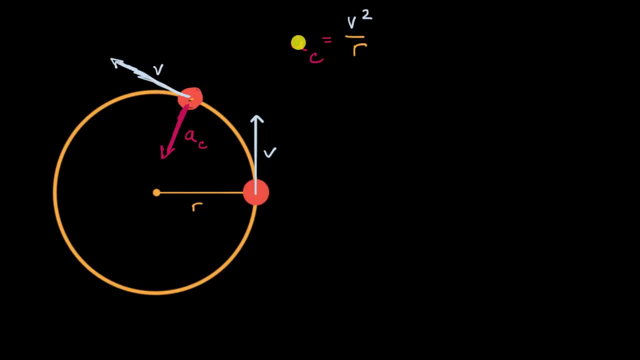 is see if I can connect our centripetal acceleration to angular velocity, our nice variable- omega right over here And omega right over here- you could use angular speed. it's the magnitude, I could say our magnitude- of our angular velocity, so our angular speed here. 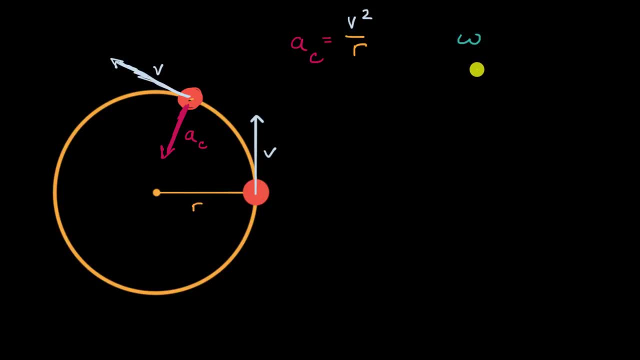 So how can we make this connection? Well, the key realization is to be able to connect your linear speed with your angular speed. So in previous videos, when we- I think it was the second or third- when we introduced ourselves to angular velocity, 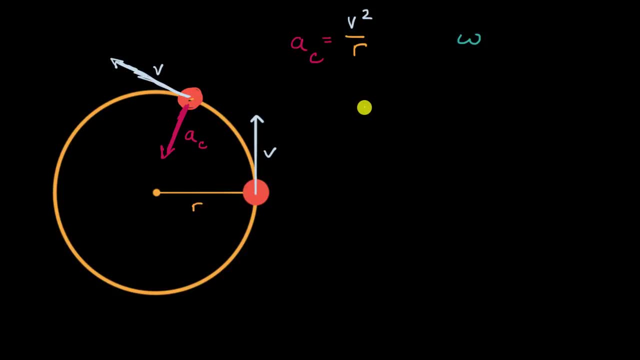 or the magnitude of it, which would be angular speed. we saw that our linear speed is going to be equal to our radius, the radius of our uniform circular motion, times times our, the magnitude of our angular velocity. And I don't like to just memorize formulas, it's all good. 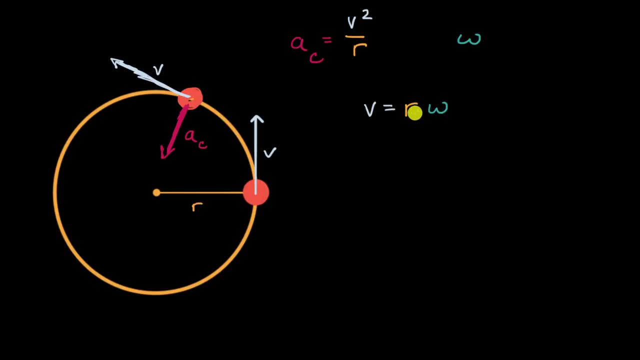 I don't like to just memorize formulas. it's all good. I don't like to just memorize formulas. it's always good to have an intuition of why this makes sense. Remember, angular velocity, or the magnitude of angular velocity, is measured in radians. 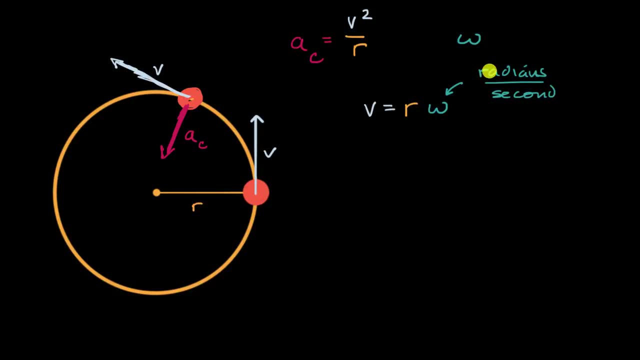 radians per second, And we typically view radians as an angle, but if you think of it as an arc length a radian could be, you could view it as how many radii in length am I completing per second? And so if I multiply that times the actual length, 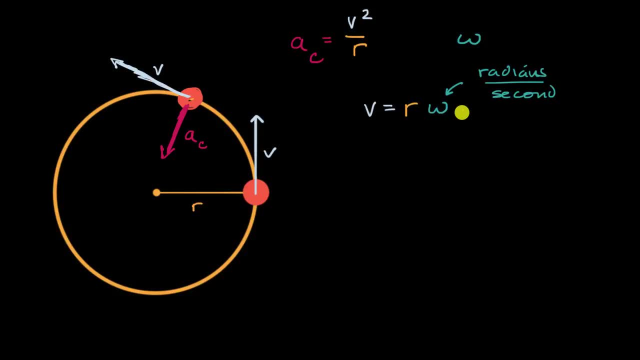 of the radii. then you can get a sense of, well, what distance am I covering per second? Hopefully that makes some sense And we actually prove this formula. we get an intuition for this formula in previous videos, But from this formula it's easy to make a substitution. 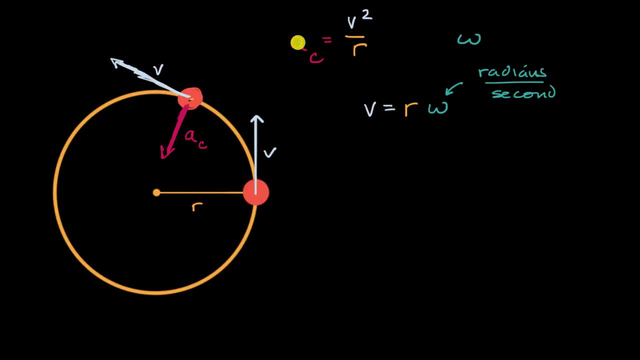 back into our original one to have an expression for centripetal acceleration, the magnitude of centripetal acceleration in terms of radius and the magnitude of angular velocity, And I encourage you pause this video and see if you can derive that on your own. 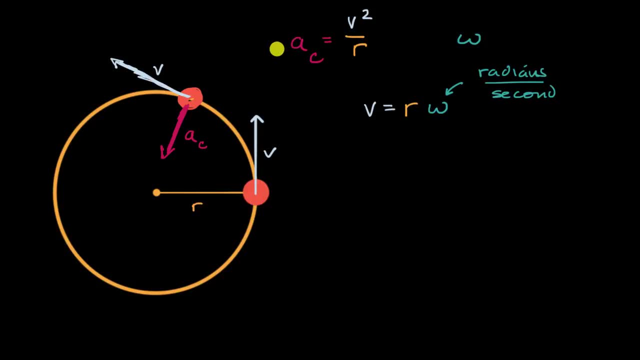 All right, let's do this together. So if we start with this, if we start with this, we have, the magnitude of our centripetal acceleration is going to be equal to: instead of putting a v squared here. instead of putting a v squared here. 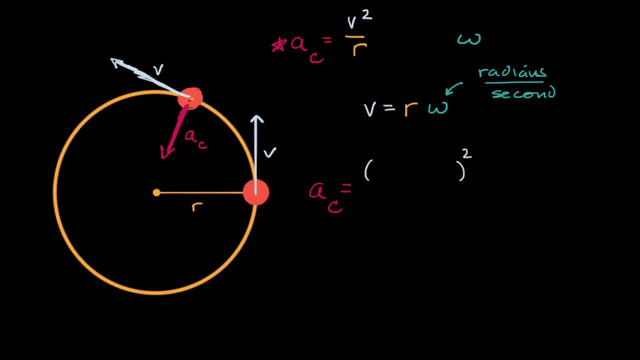 I can, instead of v, I can write r, omega. So let me do that: R and then omega. There you go, and all I did. I said: look, our linear speed right over here is equal to our radius times, the magnitude of our angular velocity. 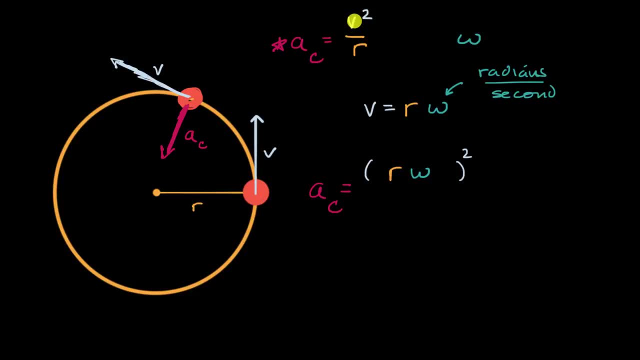 our angular speed. So everywhere I saw a v here I am just replacing it with an r omega, And so I have r omega, that entire quantity squared over r over r. and then we can simplify this. This is going to be equal to: